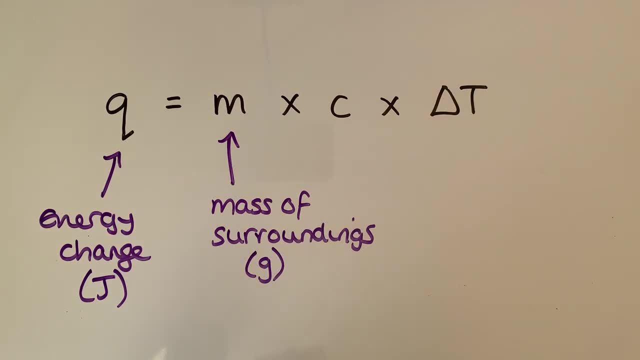 And also of the water, not the can, And if it's in a solution, you then need to work out the mass of the solution. OK, so mass of the surroundings is where your thermometer is. It's also worth knowing that if you have, for example, if your thermometer is in water and you have 100 centimetres cubed of water, 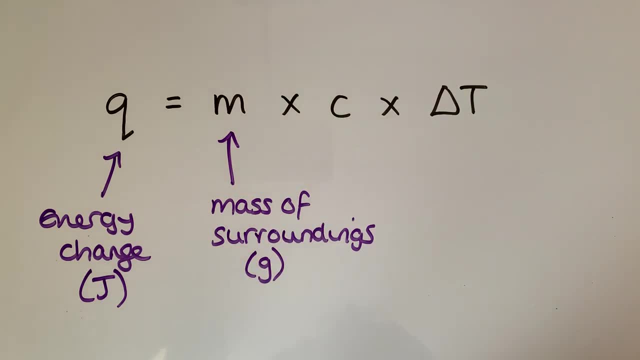 it is worth knowing that one centimetre cubed of water equals one gram. So that means if you have 100 centimetres cubed of water, that is going to equal 100 grams. The C over here is what we call the specific heat capacity. 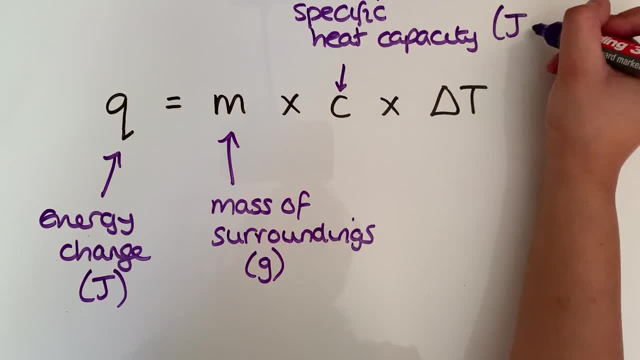 And the units for specific heat capacity are Joules per gram per Kelvin. If you haven't come across specific heat capacity before, each material has its own specific heat capacity. So, for example, water has its own value, Butane has its own value, and so on. 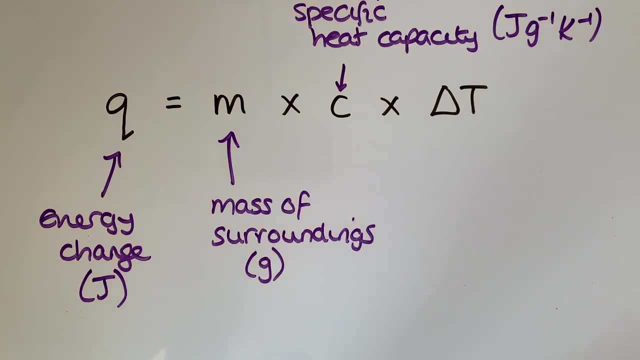 And the specific heat capacity is essentially the energy required to raise the temperature of one gram of the substance by one Kelvin. And the specific heat capacity of water is given to you in the data sheet because it will usually be of water Or they may say you know. assume that the specific heat capacity will be one gram per Kelvin. 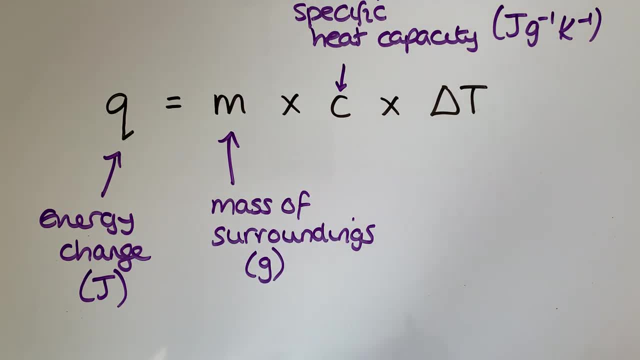 So assume that the specific heat capacity of the solution is the same as water And the value for the specific heat capacity of water is 4.18.. And, as I said, that's given to you in the exam paper- sorry, in the data sheet. 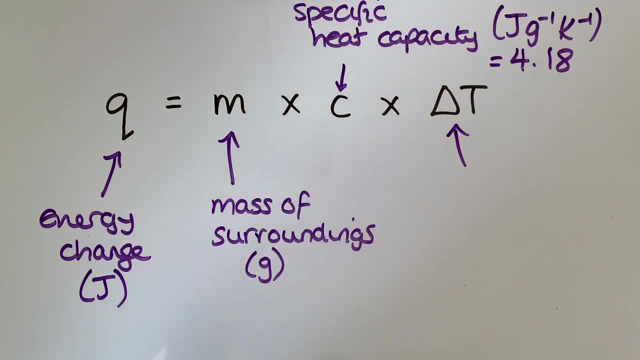 And delta T means the change in temperature. So during the experiment you know how much does the temperature change by. It's also worth noting that the temperature can go up or it can go down And essentially to work out the change in temperature you do the final temperature minus the initial temperature. 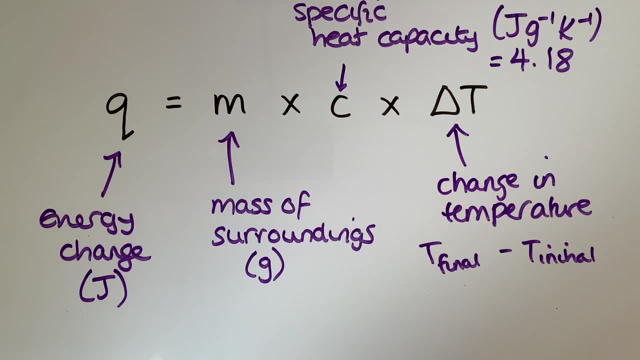 Now in terms of units. you know, in chemistry we tend to convert everything automatically to Kelvin. In this case, because you are working out the change in temperature or the difference in temperature, it doesn't actually matter whether you do this in Kelvin or you do this in degrees Celsius. 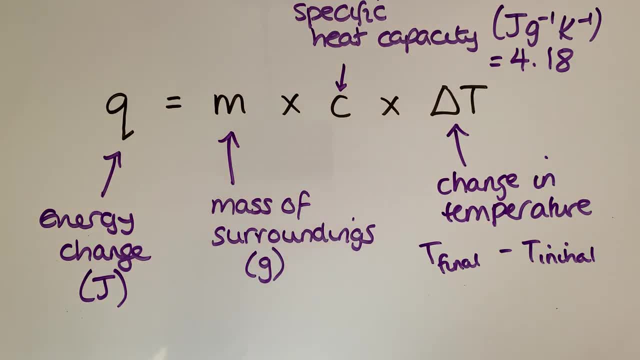 Because if you increase something by one Kelvin, it also increases by one degree Celsius, So the intervals are the same. So if I just run through kind of example of that, if I have a initial temperature reading of zero degrees Celsius and the final temperature reading is 10 degrees Celsius, 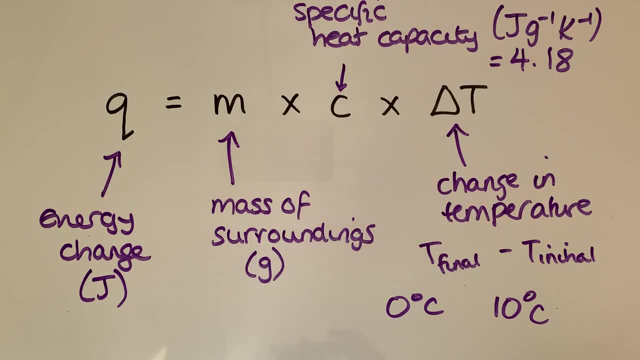 my delta T here works out as 10 degrees Celsius If I converted these to Kelvin. so to convert to Kelvin I add 273.. So this one's going to be 273 Kelvin, This one is going to be 283 Kelvin. The temperature difference here: 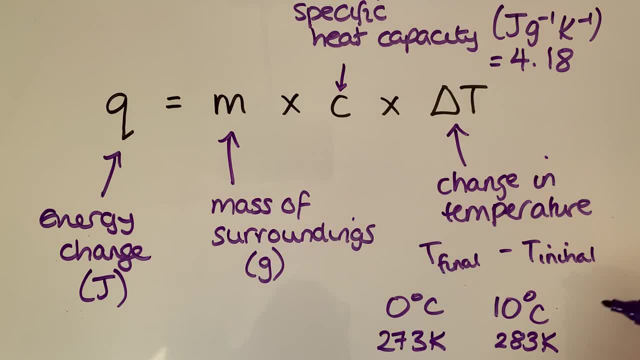 So between these two is still 10.. OK, so because we're working out the change in temperature, you don't have to waste time converting degrees Celsius to Kelvin. OK, you could just do it directly in degrees Celsius, because you're just working out the difference between the two. 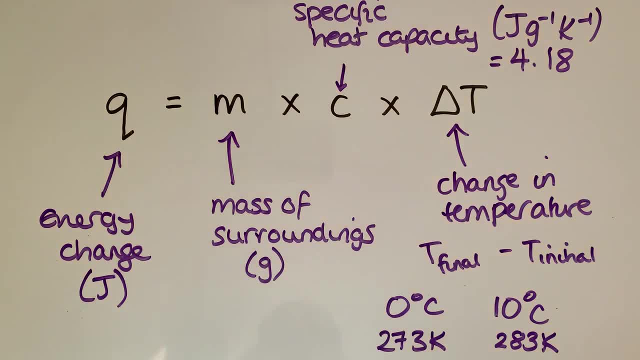 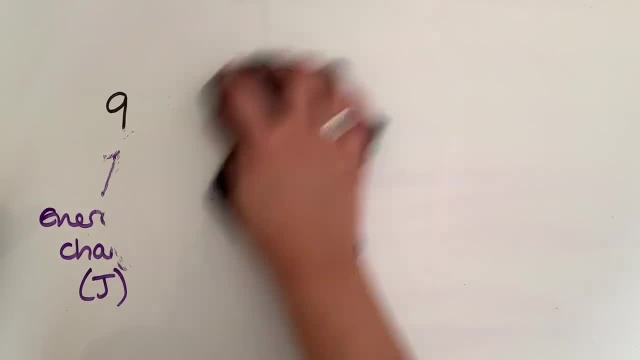 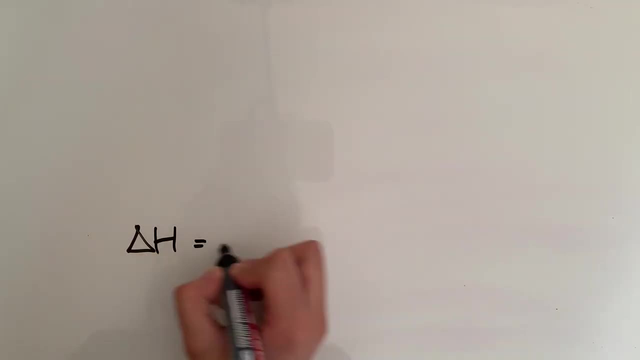 OK. so if we plug all those numbers in, we then get our Q, which is our energy change. We still haven't got to our enthalpy change Because, as we know, enthalpy change must be in kilojoules per mole. 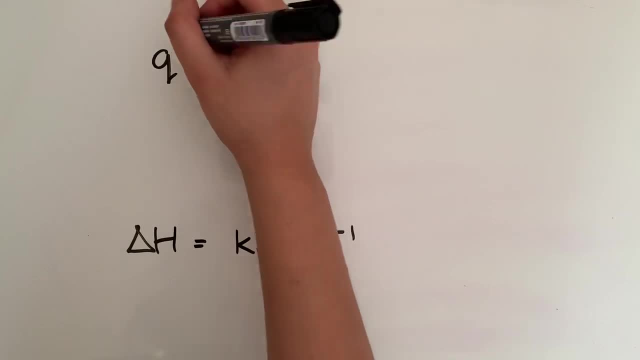 OK, at the moment we have an answer. so our Q is in joules, So we need to somehow get from our joules to kilojoules per mole. So the first thing we're going to do is we're going to divide, we're going to convert this into kilojoules. 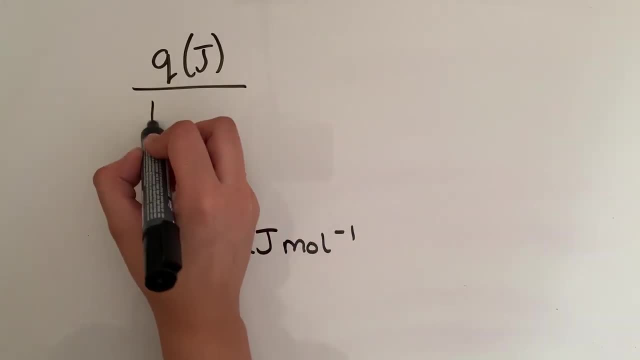 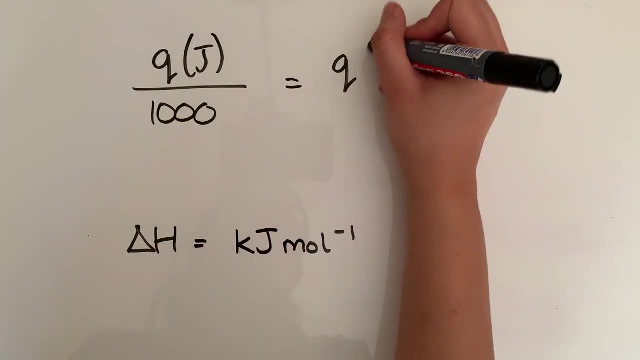 So to go from joules to kilojoules, we divide by a thousand, So that Q value that we've just got from that first equation, we divide by a thousand and then we have our answer. We still have energy change, but it's now in kilojoules. 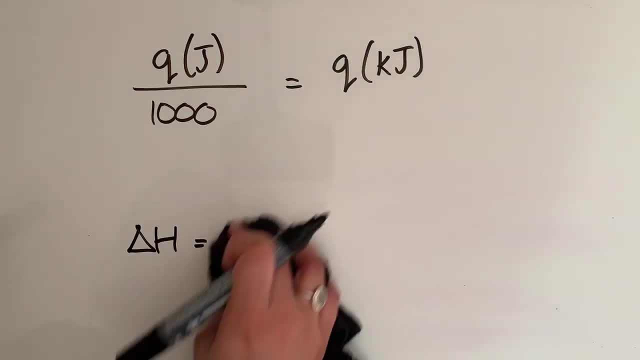 And to get to our enthalpy change, we're going to take our Q in kilojoules and we can divide it by the moles of the substance. Now, this is going to be specific to the type of experiment you're doing.